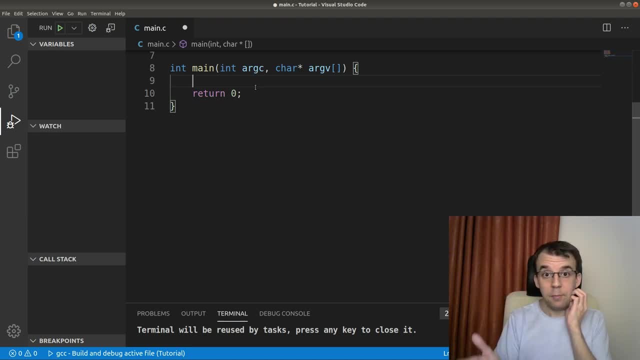 Okay, so in this case, if we want to open a pipe, what we have to do is just call the function called pipe, And this guy takes in an array of two integers. And those two integers are really important. They are the file descriptors for this pipe. A file descriptor is: 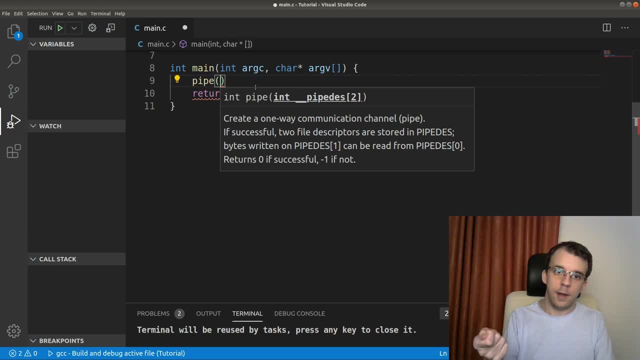 basically a key, a key for access to a file, so that we know like to, where we want to either read or write data to. So in this case I'm going to actually define here an array of two fd And this pipe function is going to save inside this array. it's going to save the file descriptors. 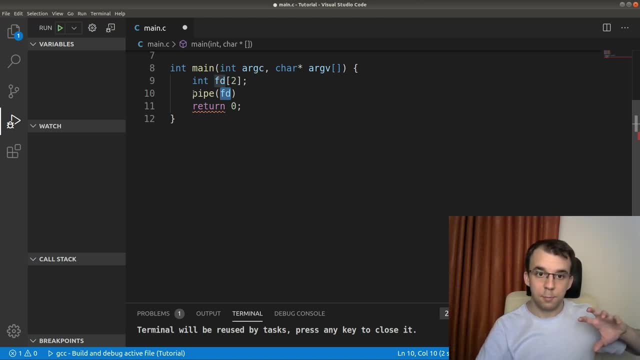 that it opens when we create this pipe, right? So this guy, this pipe function, creates the pipe And in fd we have the, basically the keys to that pipe, So we can read or write to it. Okay, So this is very similar to a file, let's say, except you get two file descriptors. 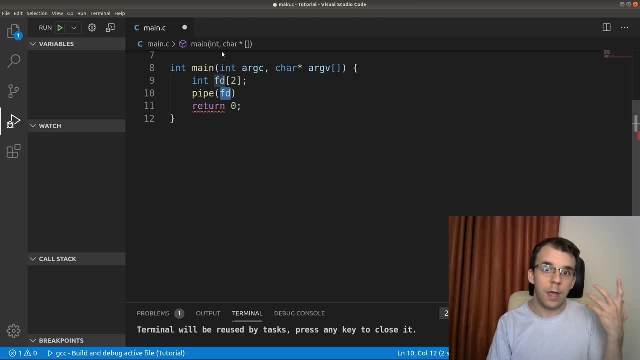 you don't only get one, So you don't. whenever we used fopen we only got one Sort of file descriptor, But in this case we get multiple And it's recommended to check if this guy actually returns zero. So if if we take a look at a tool, 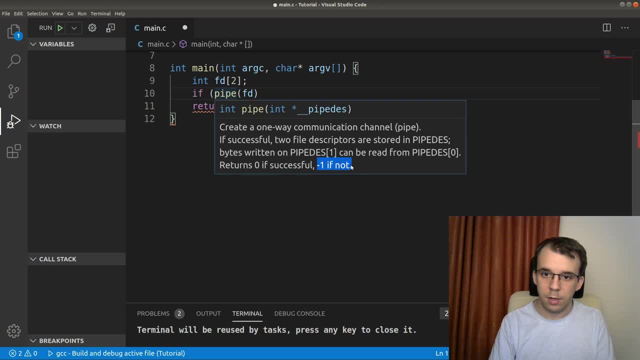 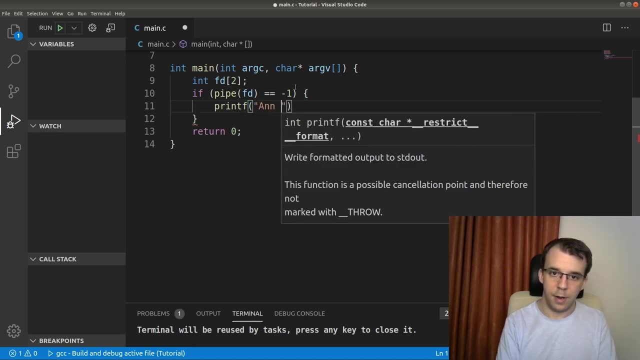 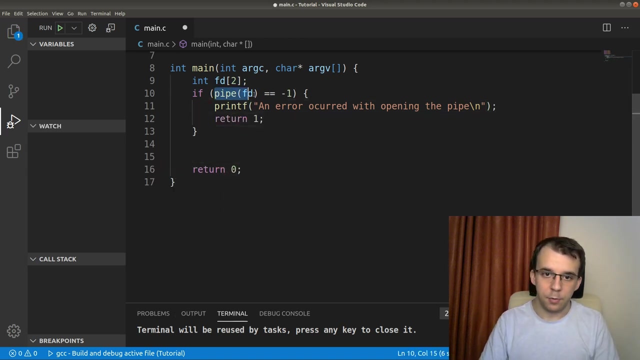 tip. it says that it returns zero if successful, so negative one. if it's not So, if we get negative one, then please do. I don't know. printf. an error occurred with opening the pipe. Let's say: and return one. Okay, so now we opened the pipe. So here we have opened the pipe. 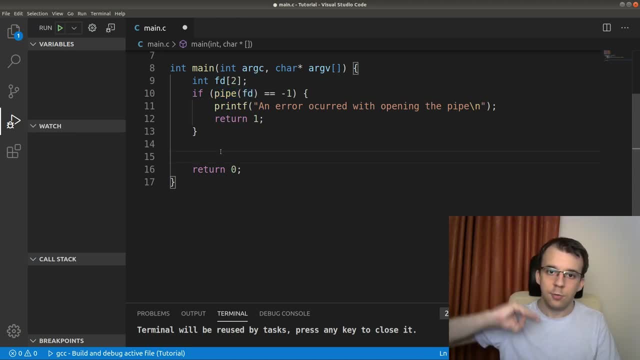 Now we can fork. Why we can only do it in this order? Well, if I say here, int id equals fork, the thing is, when you fork, the file descriptors here get copied over right. And these file descriptors are kind of nice because, aside from just getting copied, 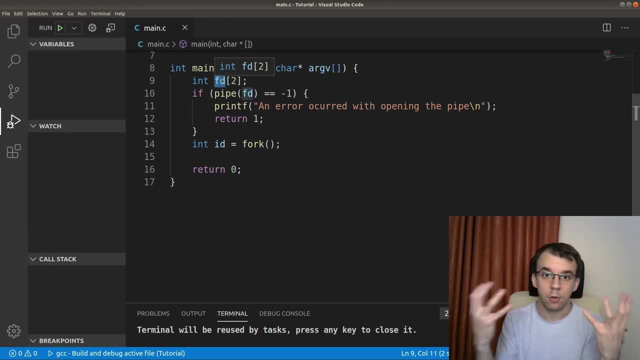 over, like only the set from those integers getting copied over behind the scenes. those file descriptors are also assigned to the new, newly created process, So they get inherited. What does that mean? Well, that means that if you, for example, close that file descriptor, 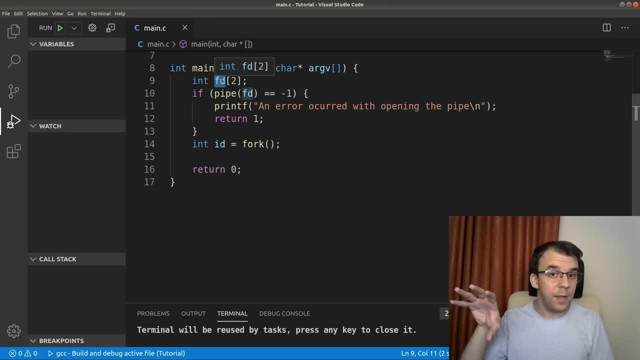 at one point in a process, well, that file descriptor in the other process remains open, So they sort of have- let's say they're independent of each other. Okay, so in this case these two file descriptors get copied over and inherited as well, So they can be. 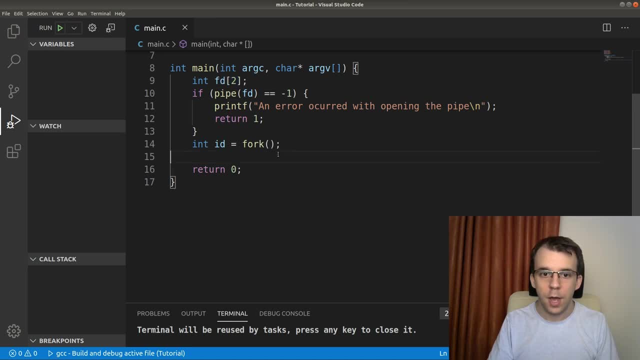 open or closed independently of each other. So now what we can do is say: if id is zero, well, what I want is just to create a simple program that what does is just asks the user to input a number And then it sends it to the other process, let's say to the parent process, from the child process. 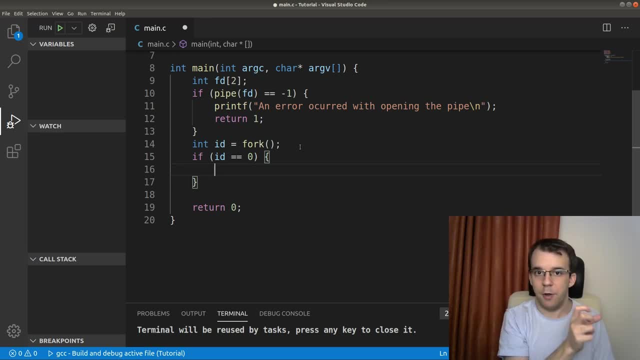 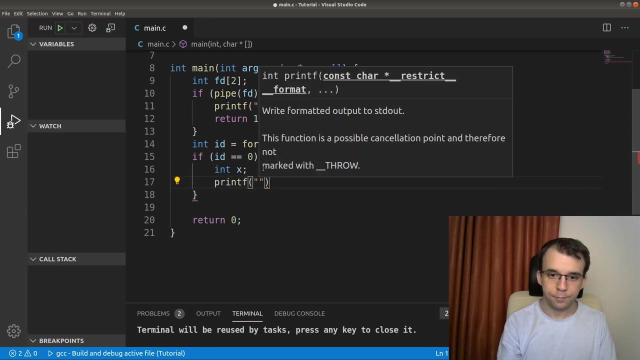 it sends it to the parent process, and that parent process- I don't know- prints it on the screen or does some operations with it. So to do so, well, we're going to have to declare here a variable. So I'm going to say int x and well, printf input, input a number. 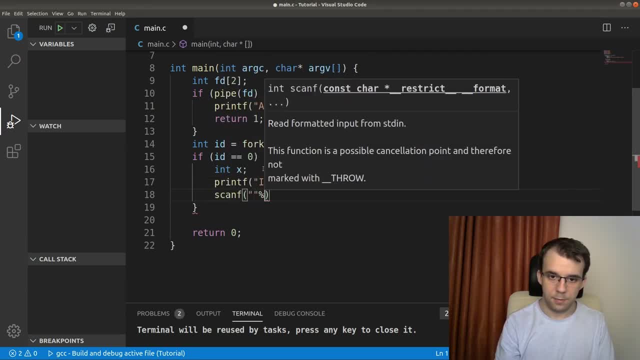 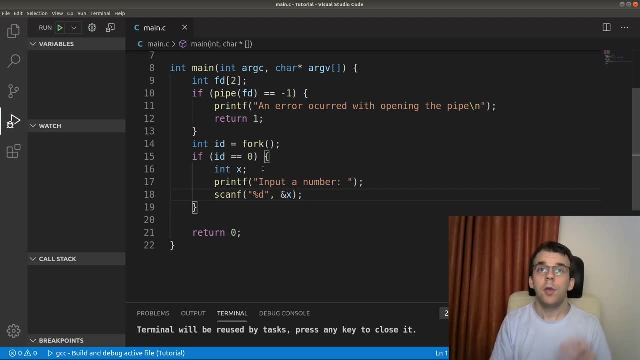 And then scanf %d and then the address of x. that's fairly standard. And now here's where it gets interesting. So we want this x to be sent from the child process. we're in the child process, right, And we want this guy to be sent to the parent process. How do we do that? 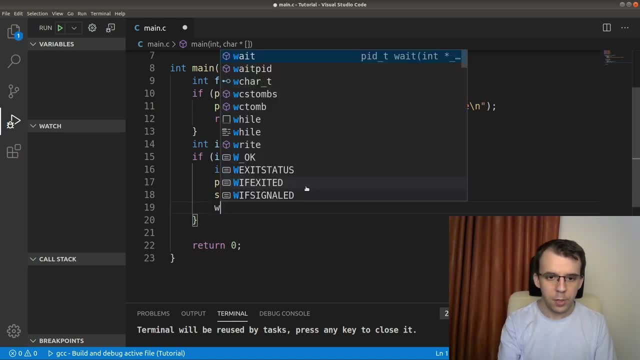 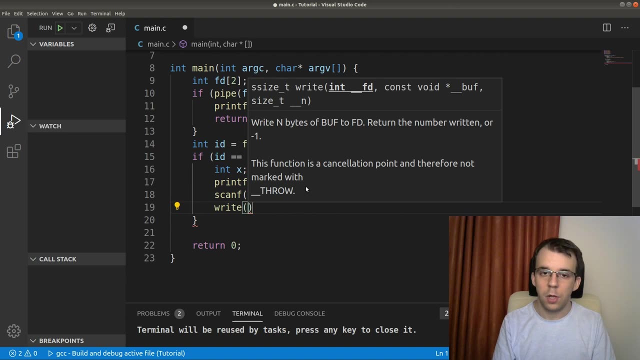 Well, there's a function called write which, by the way, you can actually use not only for pipes. you can use to write to any file. This guy takes in the file descriptor. So we have here fd of. well, I didn't tell you which is which and why do we have two here? 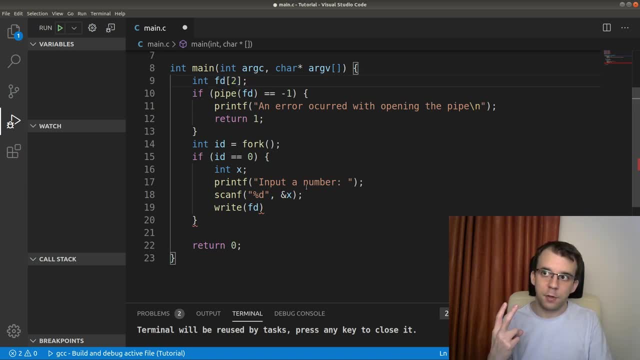 Well, here we have two file descriptors because, as the name implies, a pipe should have two ends, right? That's how a pipe works in real life. So in this case those two ends are stored in here, right. And then fd of 0 is the read end, so where you should read from, and fd of 1 is the write end. 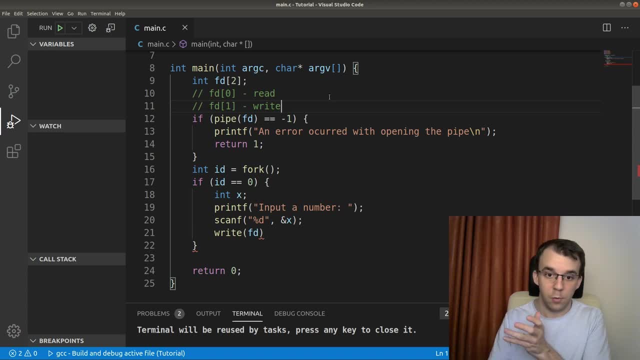 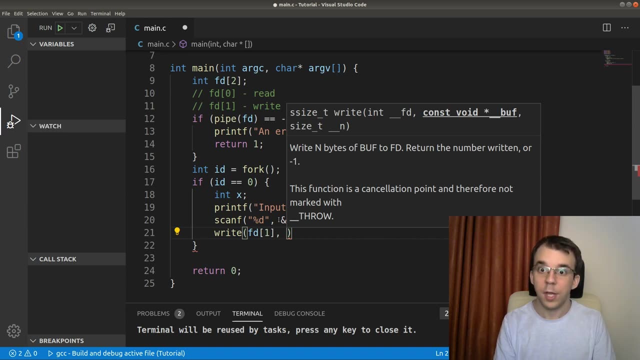 where to which you're going to write the data. So in our case we're going to write to fd of 1, and here it's telling me where to get the memory to write from. So I want to write, well, our x here. so I'm going to send in the actual address to our x and I want to write in. 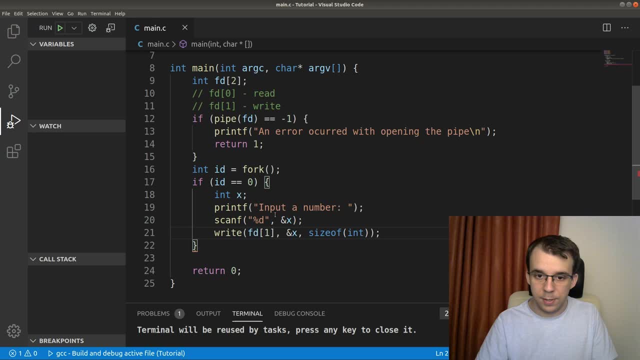 just an integer, right So size of int. that should be safe to do Next up after we're done. we're done writing. we should actually close this file descriptor, right? So like similar to how you do it with files, you just say close of fd of 1.. That basically tells: 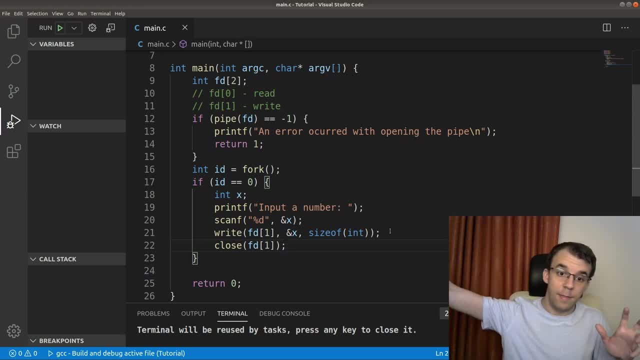 anybody that might be listening on that. on the other end, for this data, that well, this file, quote unquote, has been closed and you don't have anything to read from it. There's no longer any file descriptor that can write, that can write to it opened. So, okay, this is fine. 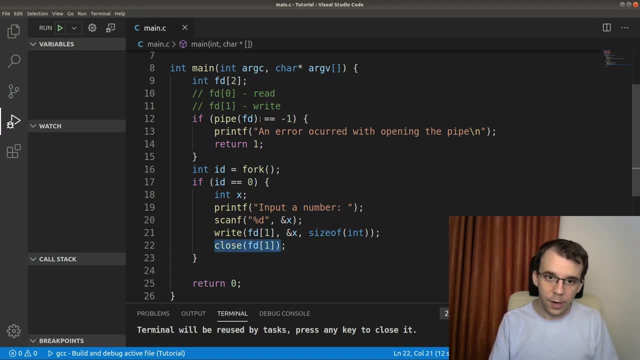 but one more thing that we have to do besides closing the right end is also close. the read ends And since the file descriptors are inherited, basically what we have to do is manage our own file descriptors in each of the process. So, since we're in the child process, 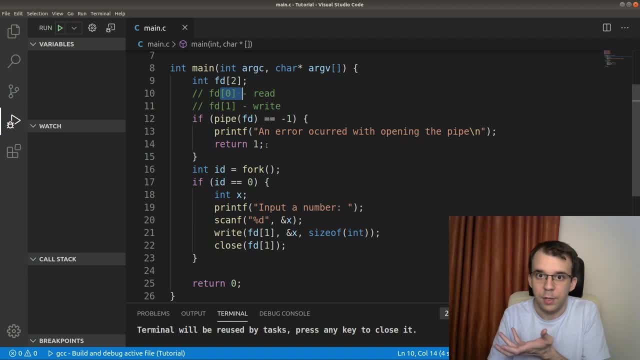 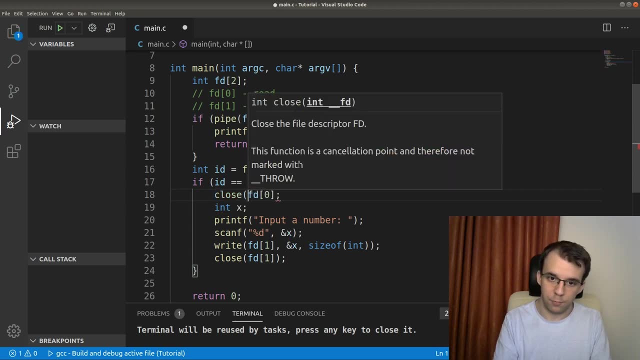 we also have to close the fd of 0, because we don't read anything from that, so we can just simply close it like right at the beginning here: fd of 0,, close of that. And this guy is a. 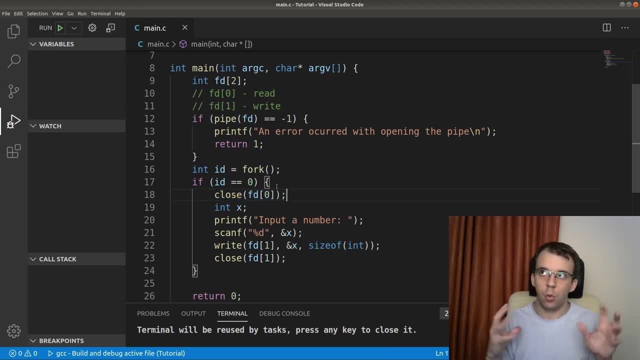 sort of standard procedure that usually you have like two. you have a pipe between two processes and you usually close one of the ends on every process, right? So in this case I just close fd of 0, because I never read inside this process from this pipe. I just write to it. okay, I hope. 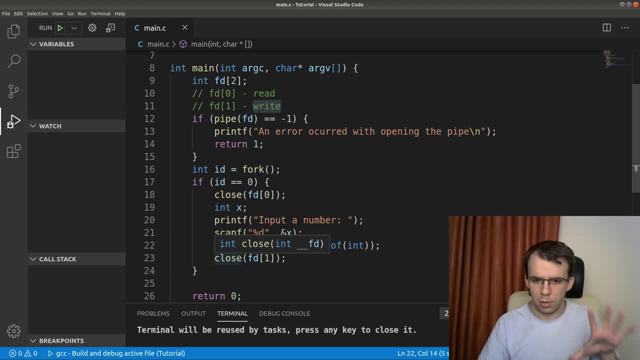 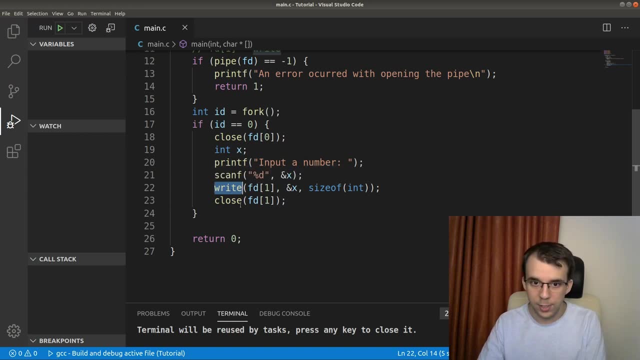 that's uh, that's sound and uh. you understood what I, what I was saying here. Now what we have to do is also read from this pipe. So, similarly, we're gonna have here an else and let's define here an int y and say: just read from again. it's not gonna be fd of 1,. 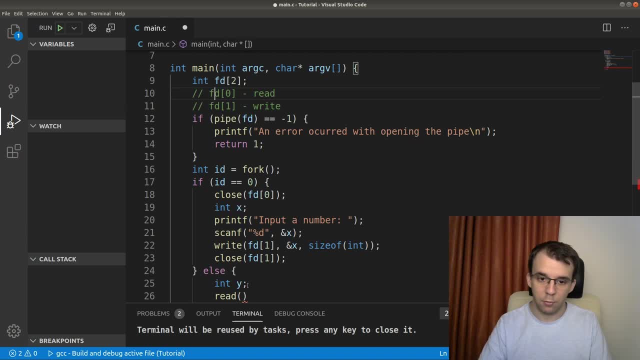 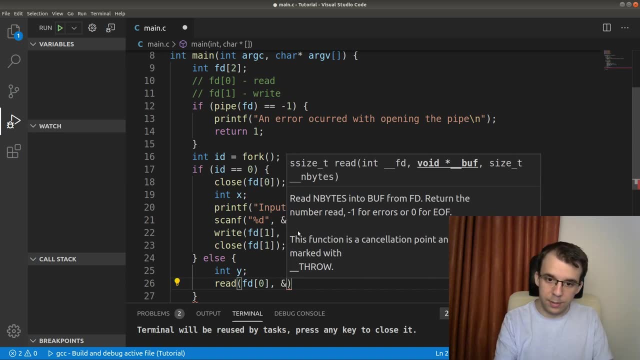 because that's the right end. so we have to actually use fd of 0 for this. I'm gonna say fd of 0, and again I'm gonna read into something: so the data is gonna be stored into y here. 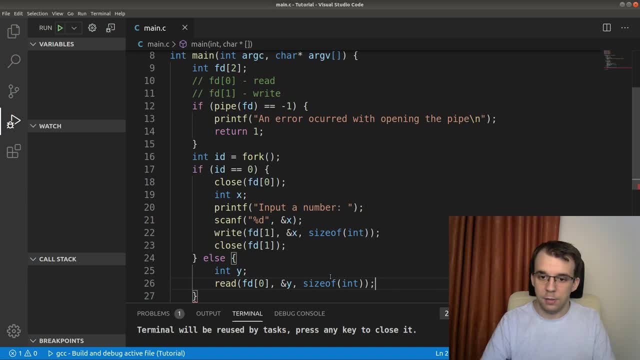 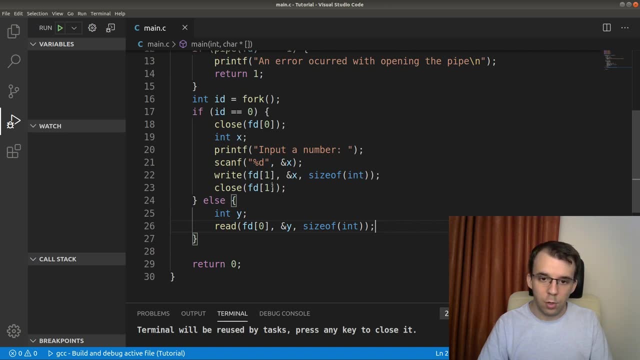 and I'm gonna read just the size of int, basically for bytes in this case. And well, as I said above, we have to close certain file descriptors. so here, since we're done reading, we should close the fd of 0, the read file descriptor, and we should also close before doing anything, the order hidden vector and so on. Uh, and that's about it. so thank you everyone for coming in today. if you find this interesting, I'm happy to answer any questions. and uh, reanimating, or you want to, some interesting all of us ideas, new material, item or interns, the uh. 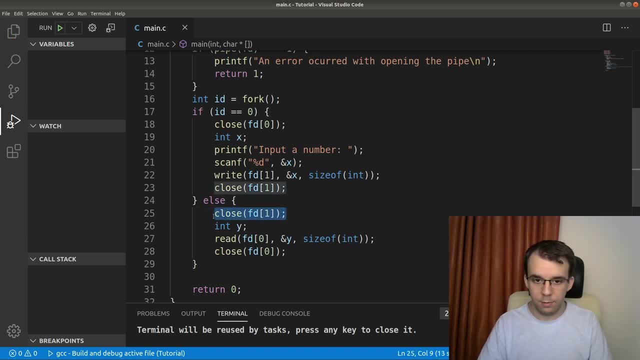 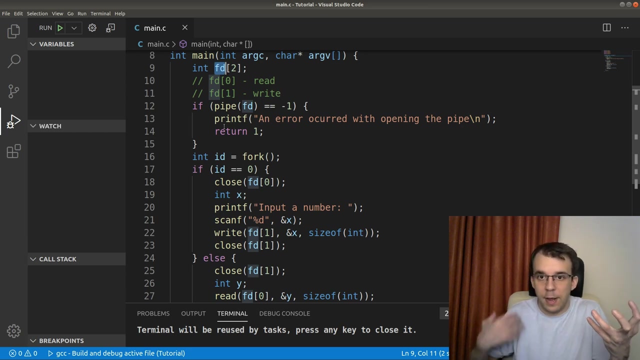 ok, question I made for everyone. If it's of interest or something else, please write it also in the comments. write descriptor, because we don't actually write to it. So, as you can see, we have four close calls because, well, we have two file descriptors but each of those two got inherited to the other. 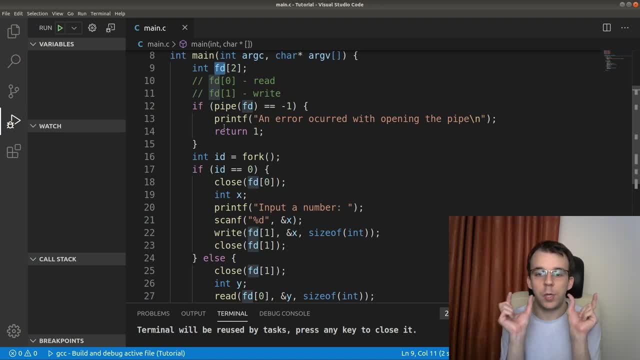 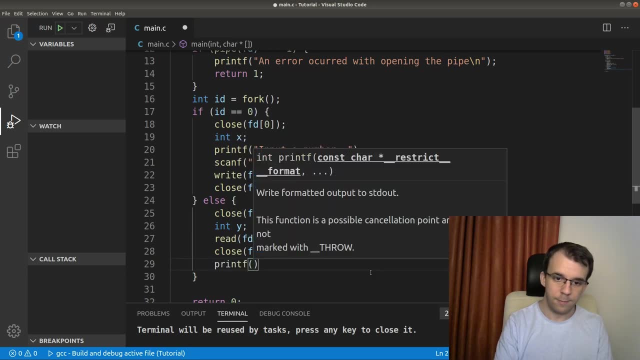 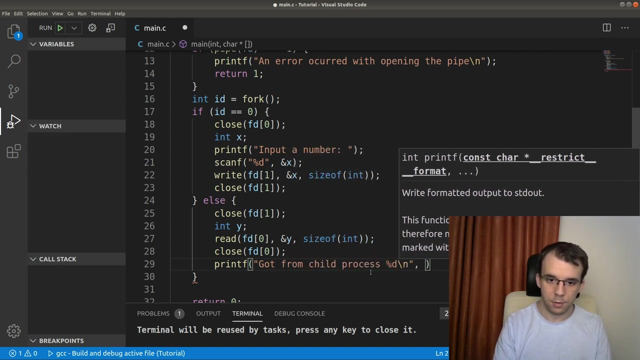 process. So we in effect we have four file descriptors that we have to close. Now, since we actually read that y value, let's actually print it on the screen. So let's say, print f got from child process, percent d and backslash d. I'm going to say here the y value. If I run this, 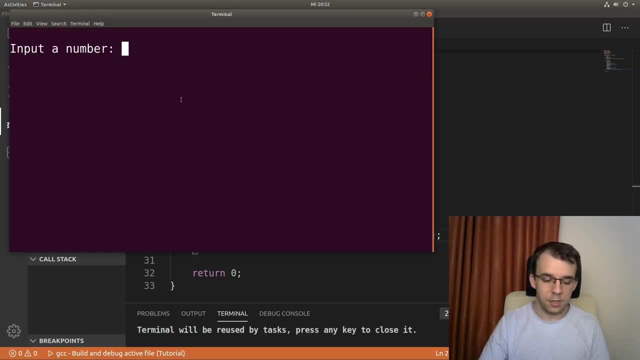 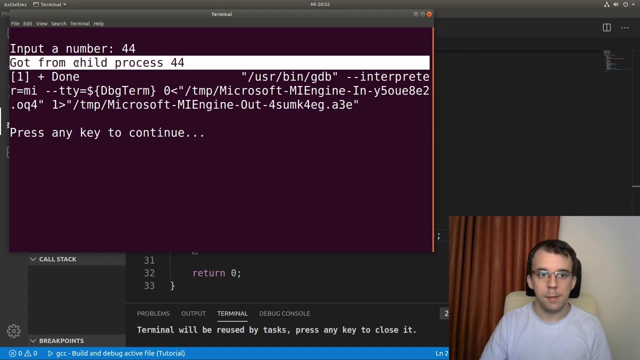 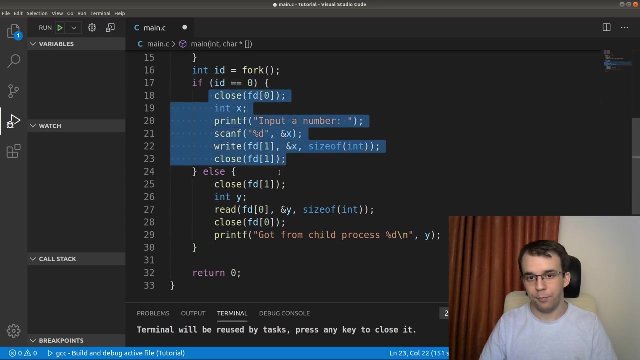 what I should get is just input a number. So I'm going to say here, let's say 44. If I hit enter, I'm going to get got from child process 44. So this is a message from the parent process, right, Remember? here id is zero. This is the code for the child process. 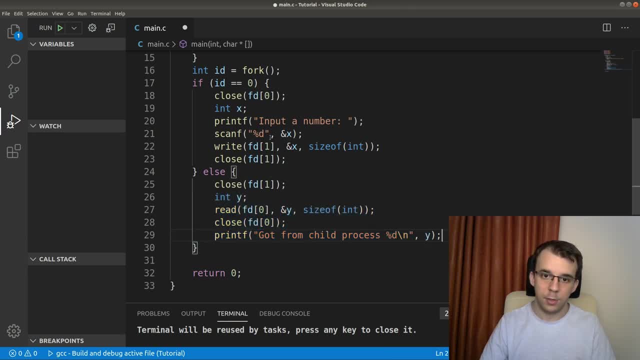 and this is the code for the parent process. Okay, so this is how we distinguish between the two. And this guy got actually written to the pipe this x here. And really this is just one integer. You can write as many bytes as you want, You just have to tell it where to sort of write. 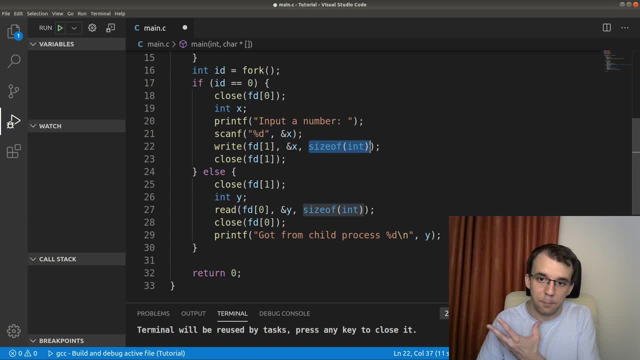 like which data? to write how many, Many bytes, exactly how many bytes. and it's just going to write that many bytes here And on the other end, it's going to read that many bytes into this address here. It doesn't matter if it's an. 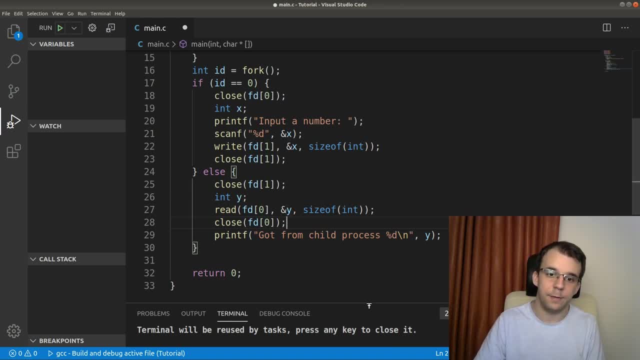 int. if it's a char or whatever, it's just going to actually plop it in there. All right, so this is how all works. One more thing before I stop the video here is you should check for errors whenever you write or read data. So here: 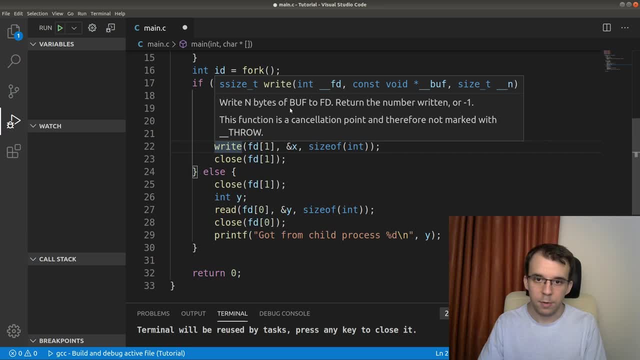 this write guy. if you actually hover over it it's going to say write and bytes of buff to fd. return the number written or negative one, And negative one means there was an error, something really bad happened and we should actually treat this. So we should say probably. 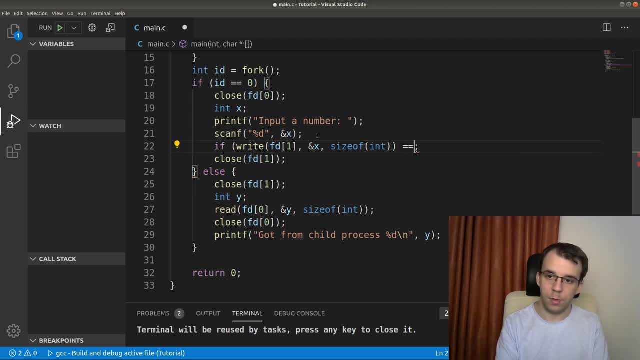 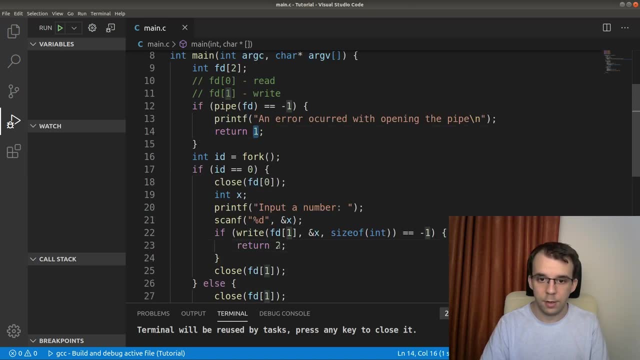 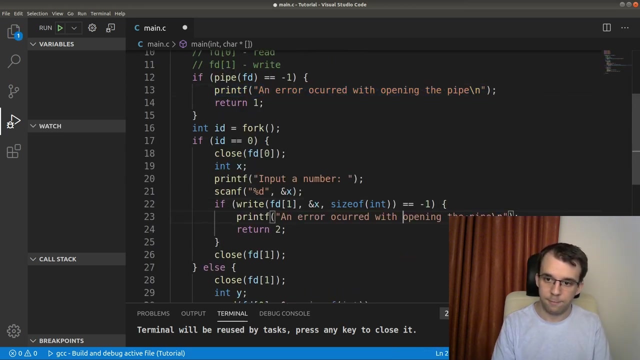 something like: if write is negative one, then let's actually return something like two. I'm going to return two because it's different than the one here, and it should be pretty obvious that something bad happened. We can also type in a message saying that an error occurred with writing to the pipe, for example, And 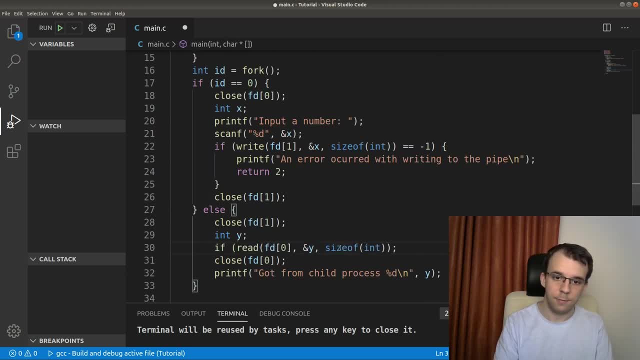 similarly when reading. you should do this. You should say: if read of that is negative one. if I actually hover over it, it's going to tell me that negative one means something really bad happened and zero means that we got the end of file descriptor. Now if we go here, we just 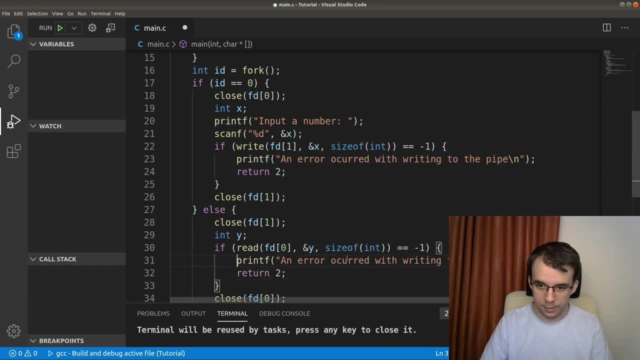 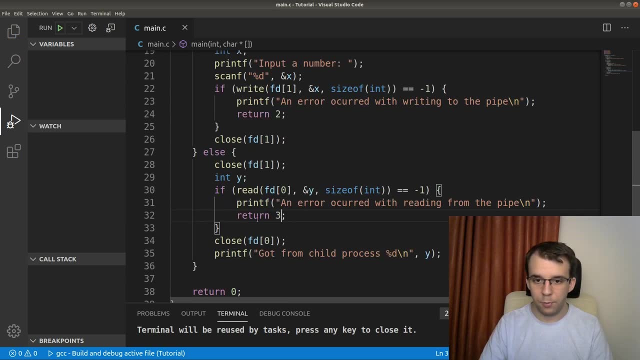 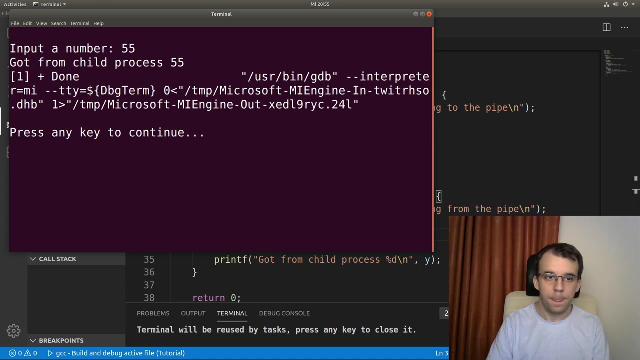 copy this over to here. Let's say something like with reading from the pipe, and then I'm going to return three here And of course the code is going to work the same way here. If I launch this, I'm going to say I don't know 55. We're still going to get 55. And of course we can do any. 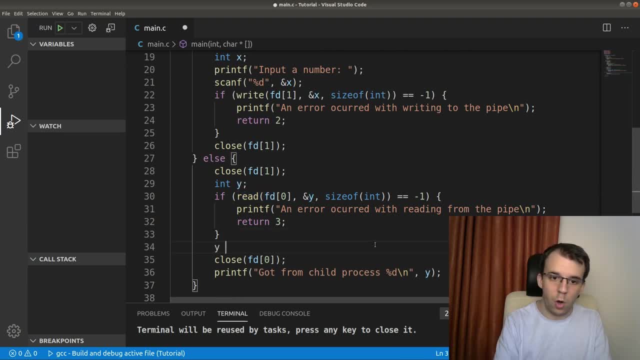 operation with this. Once we read it from here, we could just say y equals. let's say y times three. Why not? If I run this, if I, for example, type in 10, I should get 30.. And since we added error checking. 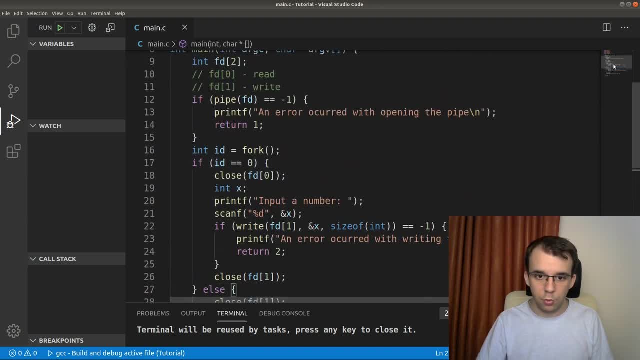 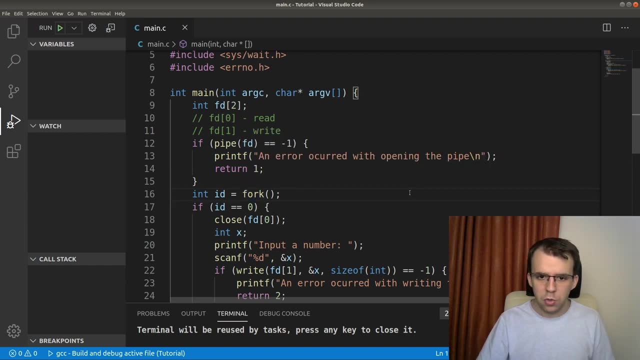 everywhere in the program here. I really suggest you actually do so when forking as well. So fork can actually return negative one if it couldn't create a process. So we should probably treat this as well So say, if id is negative one, then something like with: 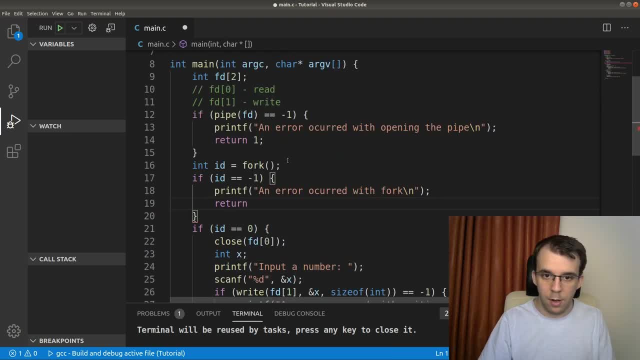 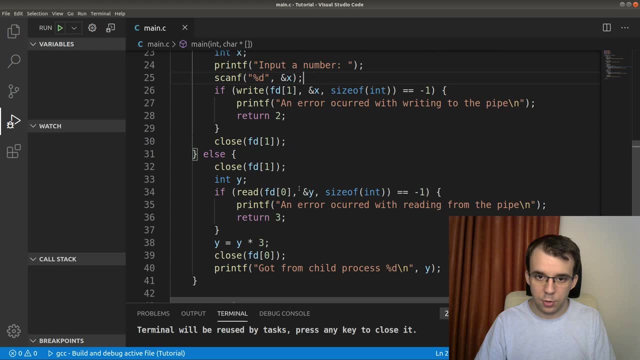 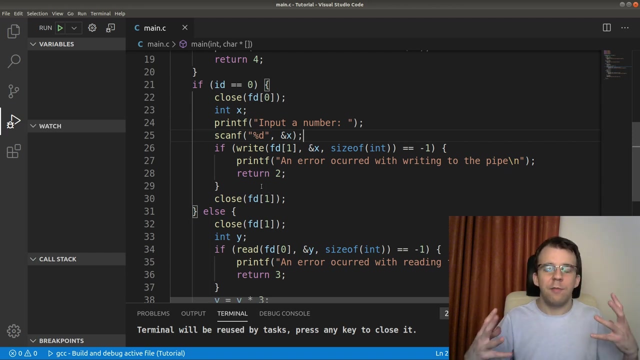 return four, let's say. and then we're going to return: well, return one here. we returned two, three, so this should be four. It's, it's a nice way to actually keep them different here And now. if we, if we check everything for errors, then when something breaks you're going to figure it.